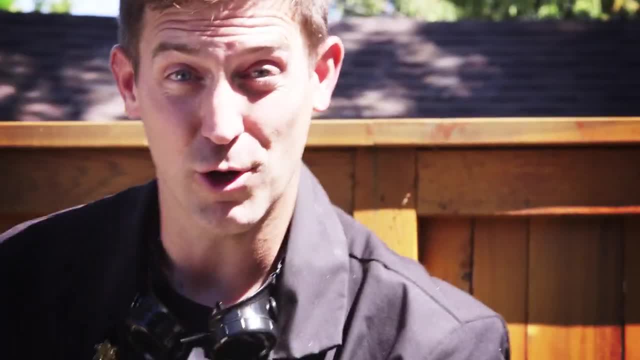 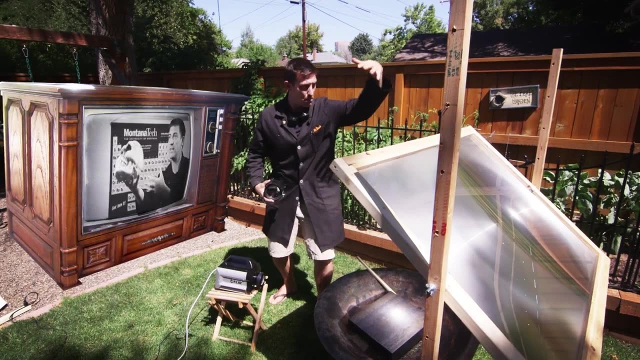 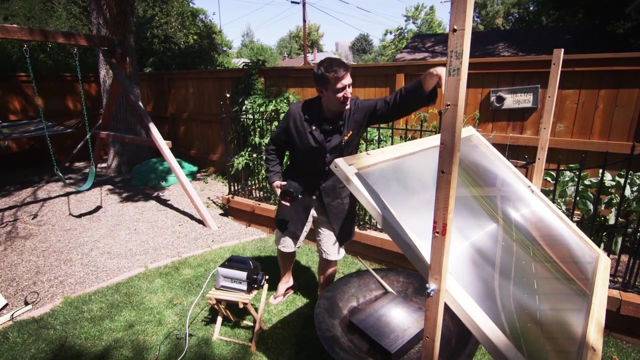 with a magnifying glass this size, imagine what you could do with a massive one like this. So this is a Fresnel lens. This is off of the front of a 51 inch big screen TV, So I've got the sun up high. it's a beautiful day: 90 some degrees, and it's shining down. 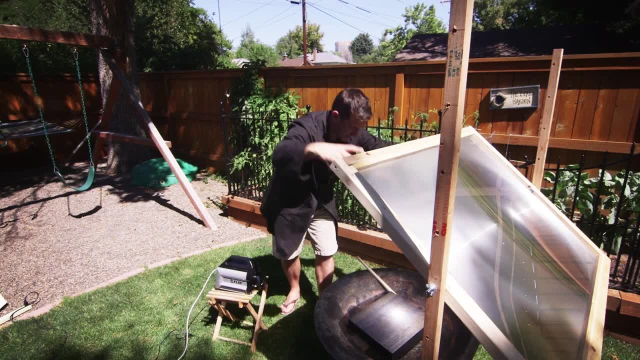 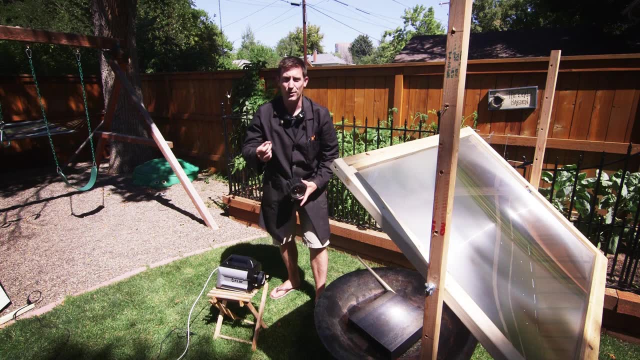 And now this is focusing- just like it did with this- into one spot down here. So it's taking all of that energy and pounding it into this steel plate. What we're going to try to do today is put some things in that beam of light and see what happens. This is: 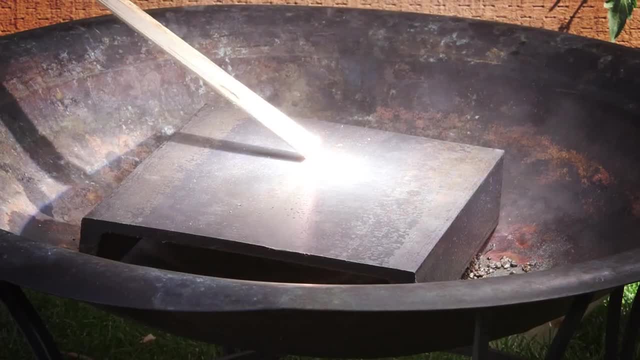 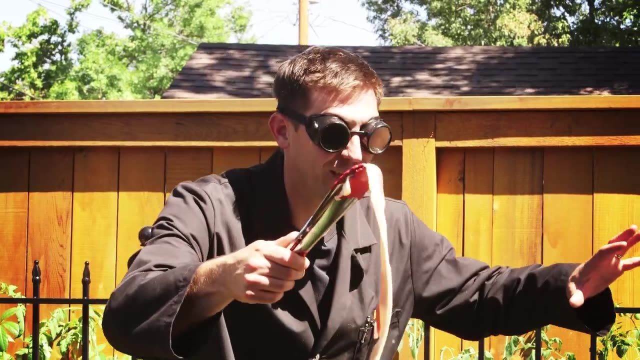 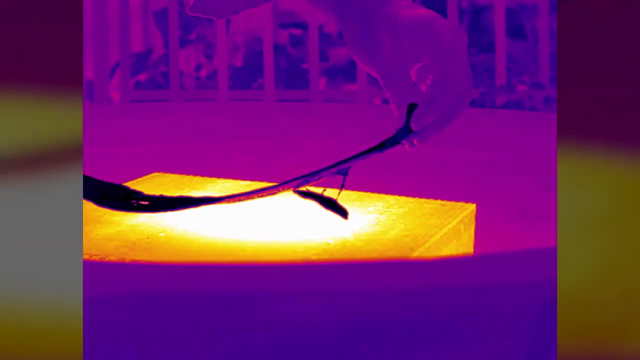 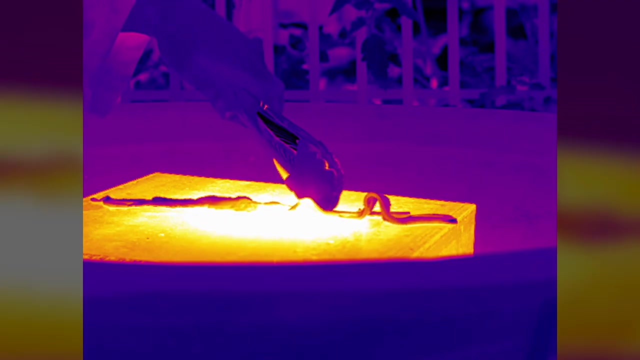 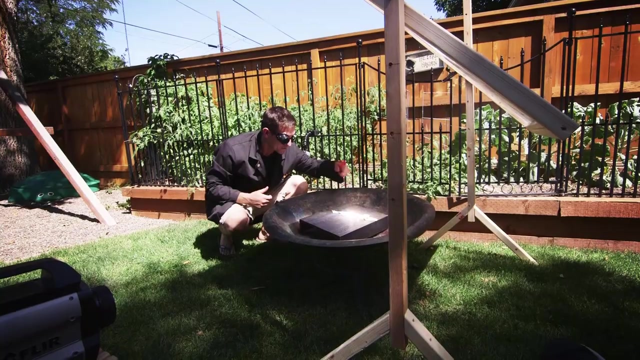 amazingly bright. One, Two, Three, Four, Five, Six, Seven, Eight, Nine, Ten, 11, 12, 13, 14, 15, 16, 17, 18, 19, 20, 21, 22, 23, 24, 24, 25, 26, 27, 27. 28, 29, 30, 31, 32, 33, 33, 34, 35, 36, 36, 37, 38, 39, 40, 41, 42, 43, 44, 45, 46, 47, 48, 49, 50, 51. 52, 53, 53, 54, 55, 56, 56, 57, 57, 58, 59, 60, 61, 62, 63, 63, 64, 65, 66, 67, 68, 69, 69, 70, 71, 72. 72, 73, 74, 75, 76, 77, 78, 79, 80, 80, 81, 82, 83, 84, 85, 86, 87, 88, 89, 90, 91, 92, 93, 93, 94, 95. 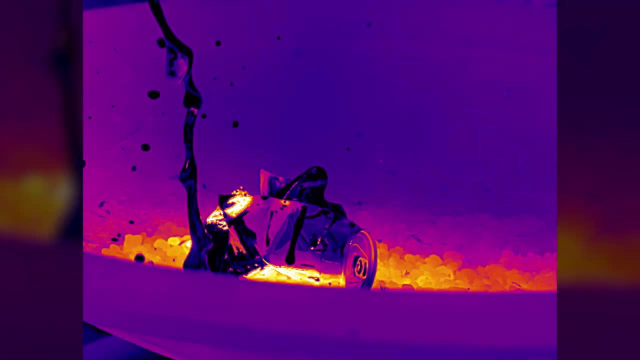 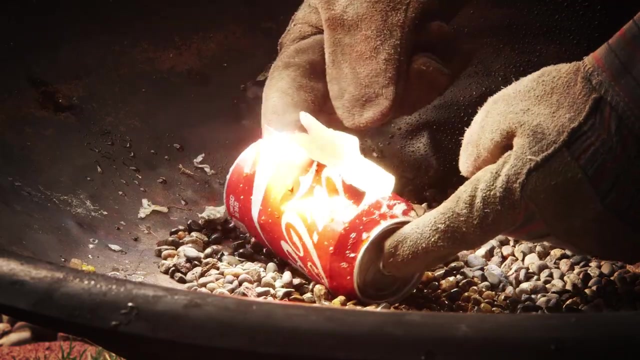 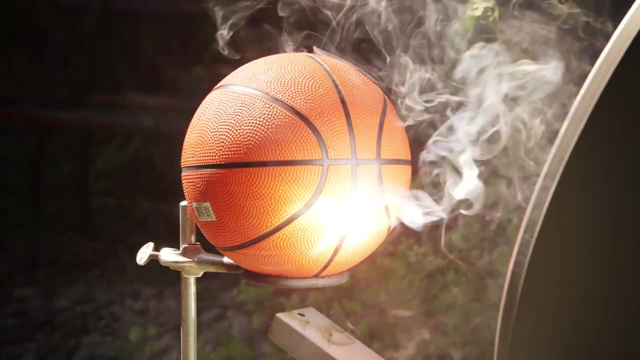 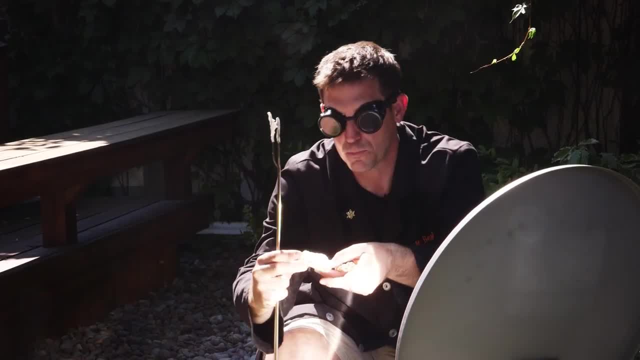 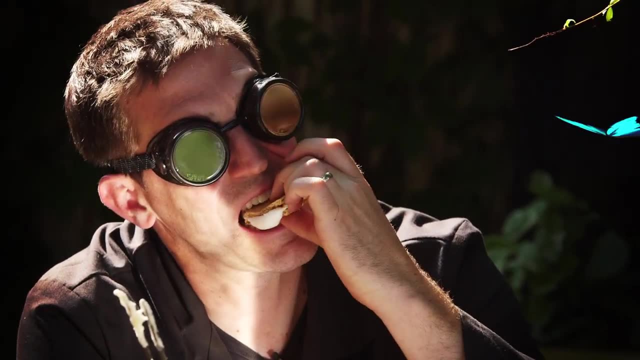 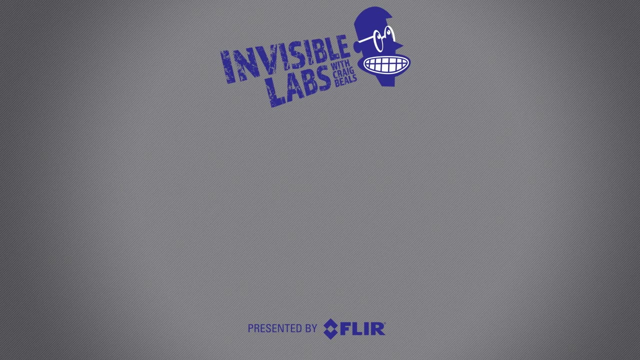 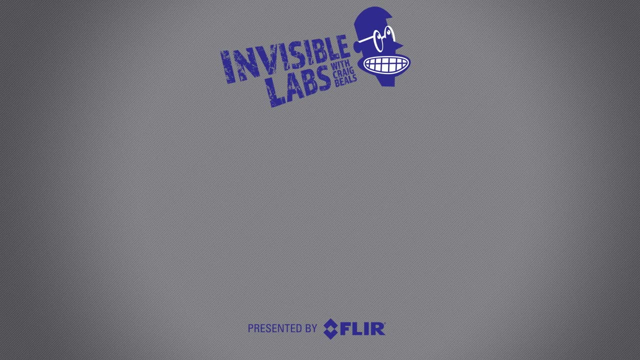 click on subscribe or come on over to the channel and check out all the amazing things that infrared is showing us.